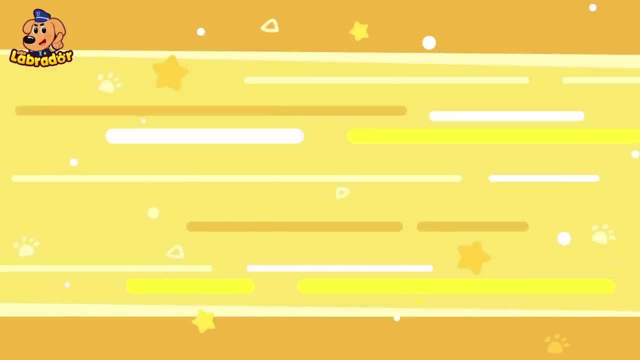 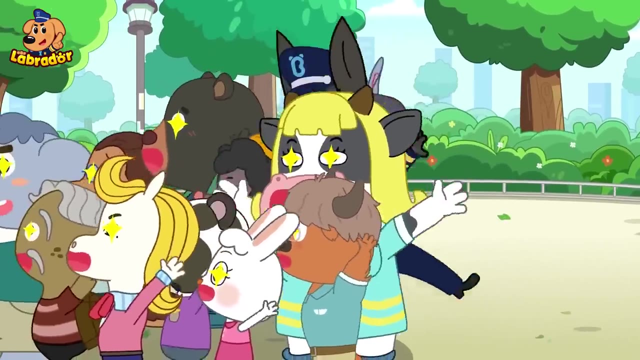 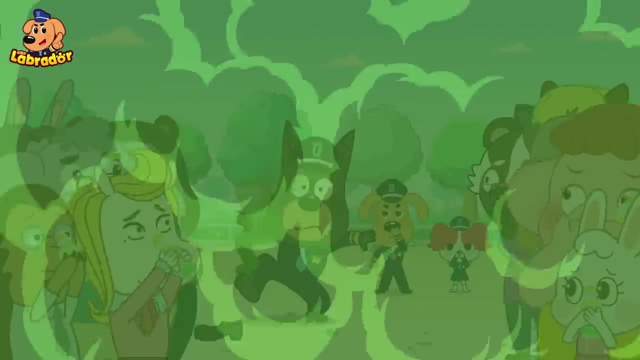 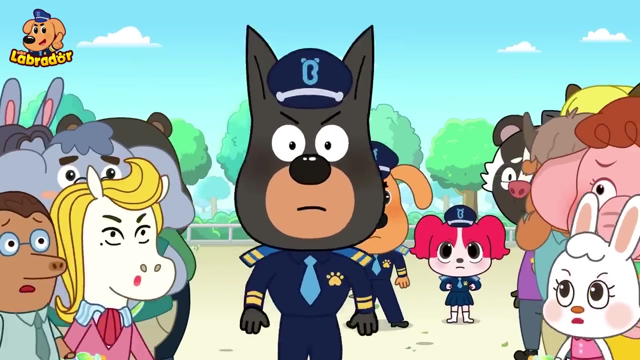 Something's wrong. Let's go have a look. I'll go buy one. I'll go buy one. I'll go buy one. Excuse me, It stinks. I lost my shoe. Police. Thank you for your cooperation. Papillon check the drink. 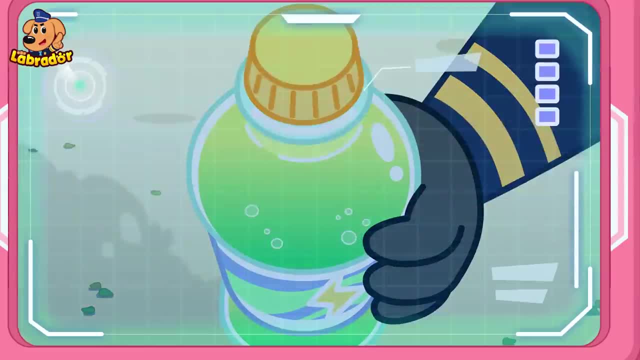 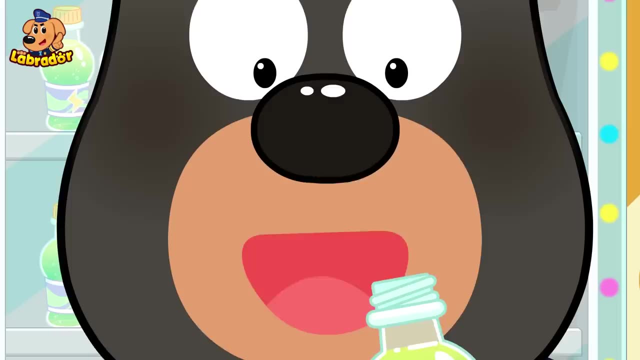 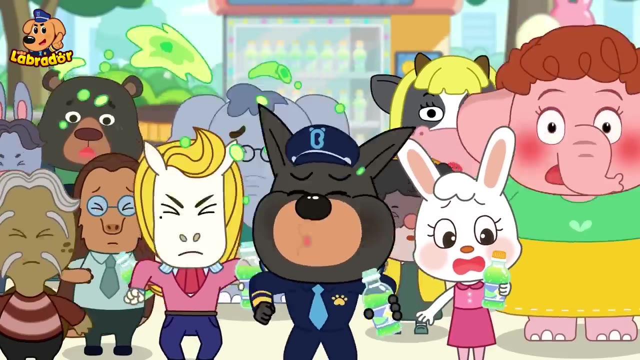 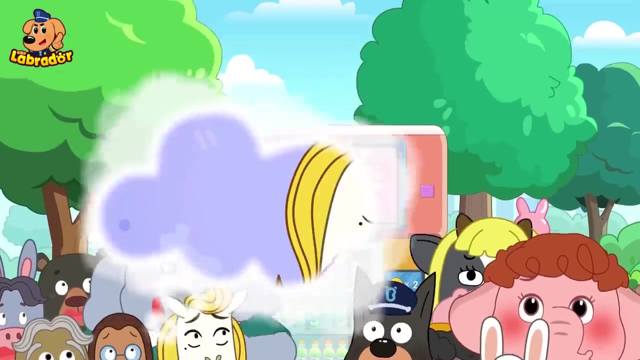 Okay, It smells great. I'm going to take a sip. Stop. Something's wrong with the drink. Look, It contains a lot of unhealthy stuff. They might make your hair fall out or make you bloated. Oh, Oh, Oh. 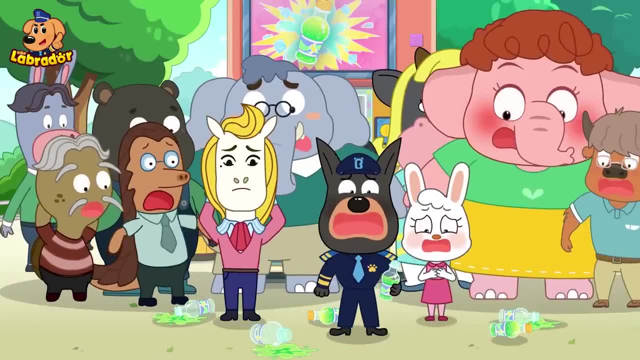 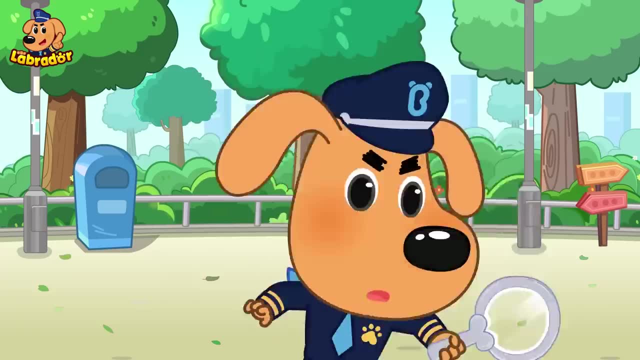 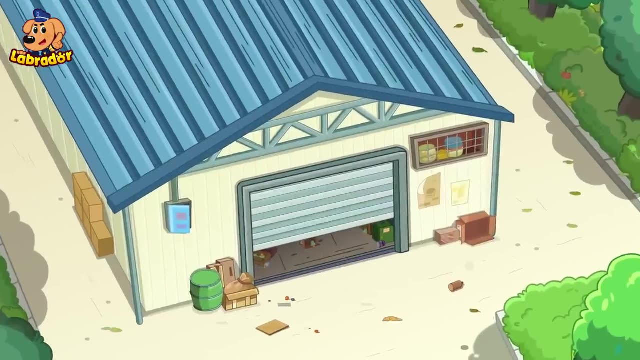 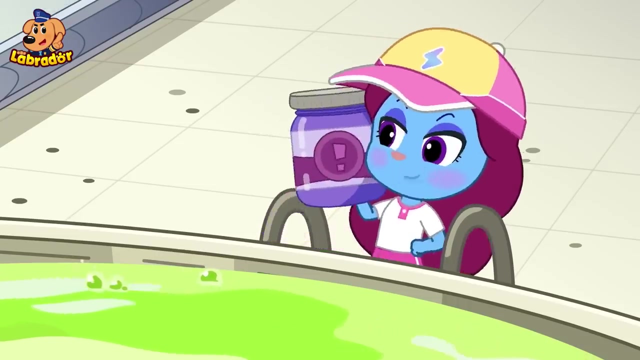 Oh, Oh, Oh Oh. Everyone stop drinking it. Who made this drink? It's horrible, Don't worry. There's no case that I can't solve With my special ingredients. people won't stop drinking it As long as I can make money. 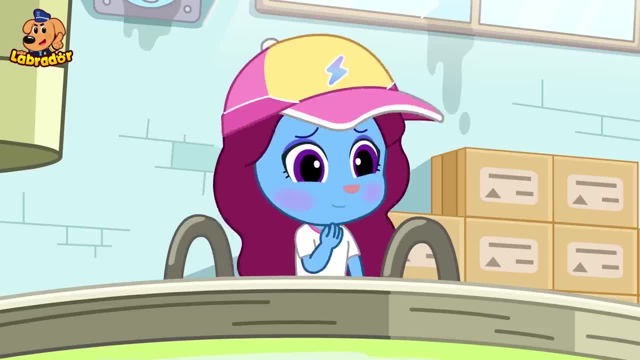 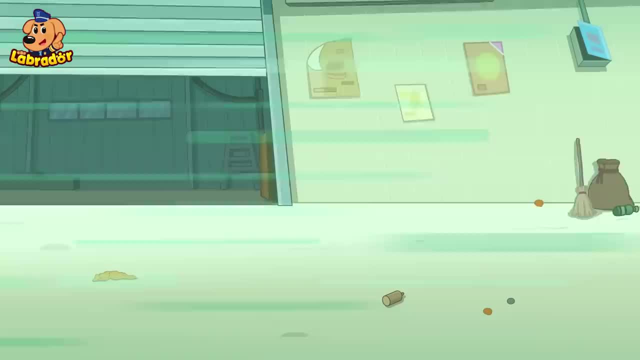 I don't care if you lose your hair or become bloated, I'm going to buy you a big pot of beer. That's not fair. Oh, That's a good idea. I think we should go to the store. Oh, There's a flask. 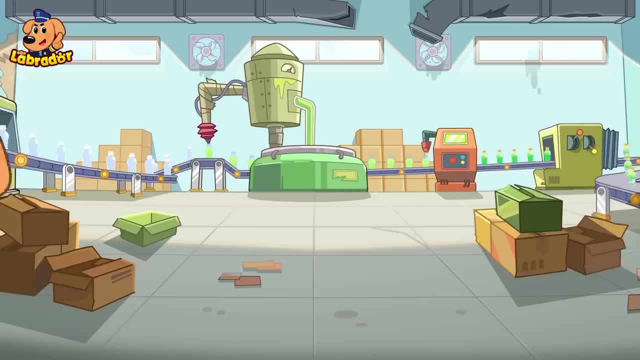 Oh my gosh, It's a bottle of beer. I can't believe this. You can't say that, can you? Oh good, It's just a bottle of beer. Oh, it's in a bottle. It's in a bottle. 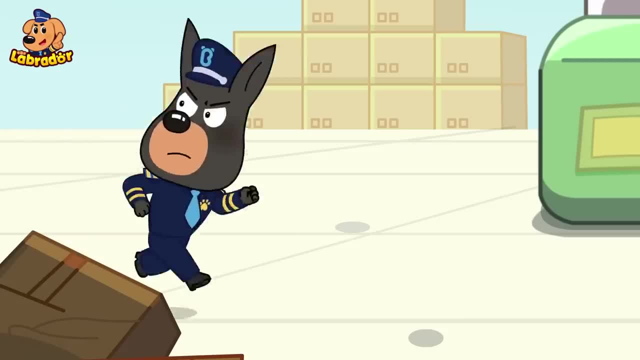 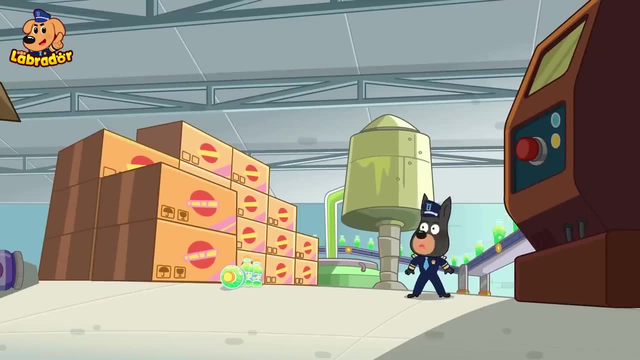 Oh, it's in a bottle. Here you go, kiddo, Here you go. Thank you, babe. Thank you, Here you go, Here you go. Huh, That's strange. Where are they hiding? What are these strange things?